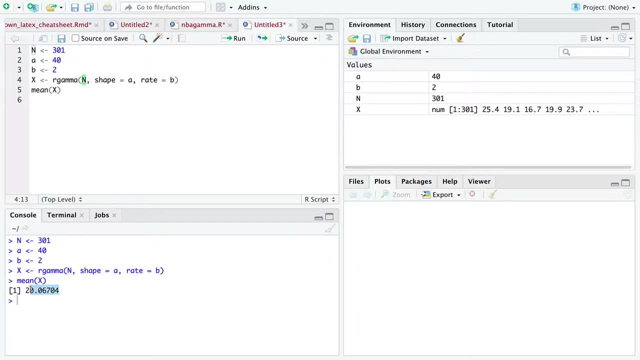 length 301.. And the mean of that vector is roughly 20, fairly close to A over B. Indeed, as the estimate from data alone is supposed to estimate the expectation. If you don't know where I got this, just Google it and pull up the Wikipedia page for the shape and rate variation. 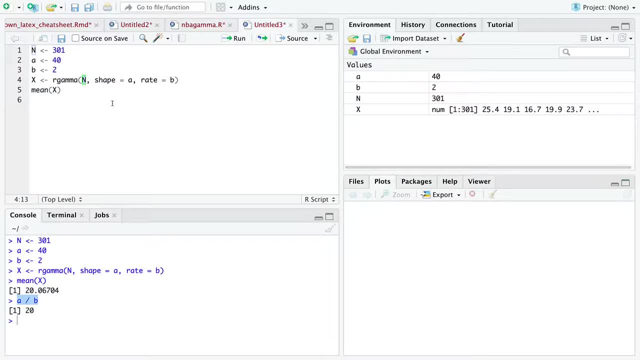 of the gamma distribution. Now, the only thing we need to really change here is to somehow repeat this process capital R times. So all I'm going to do is say that I have 503 friends And I want to do this entire process 503 times, So I've run this code just a few more. 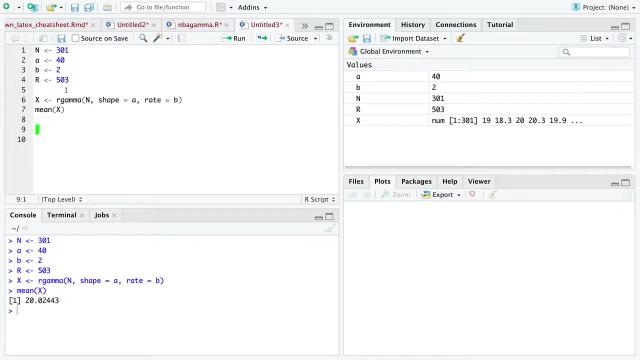 times, just to make sure I've got it all down. And here's what I'm going to do. in order to replicate, that is, just repeat This code- I'm going to use the function replicate that takes the first argument, R. 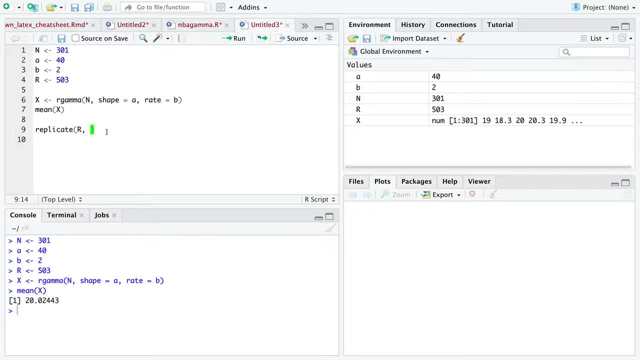 to tell you how many times you want to repeat the following expression. And then I'm just going to collapse this down into one line of code, So I'm going to call the mean. Now I'm going to try to use spaces here to help your eye see the parentheses going on, So I'm going to call the mean. 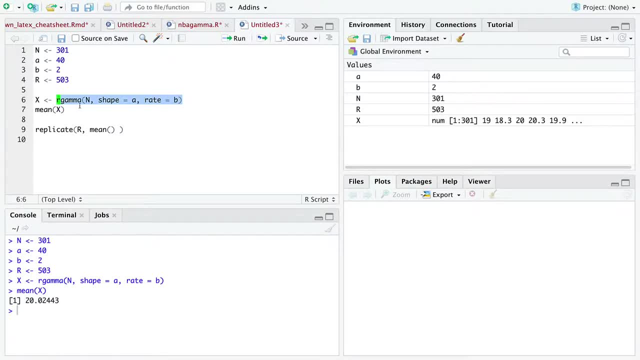 require a plus one like 16, times all, because it does the same thing If I hit all the way to the bottom, So see how tall this is right there. So I'm going to remove it right here and then do the same thing. 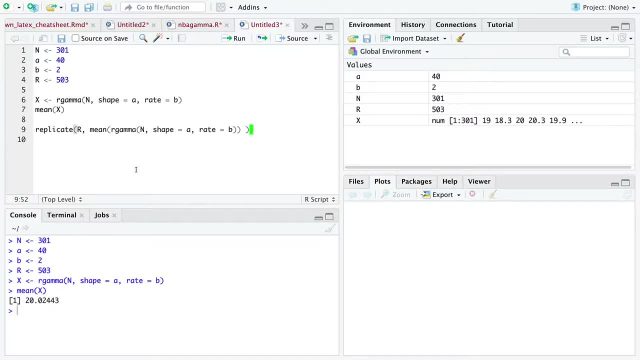 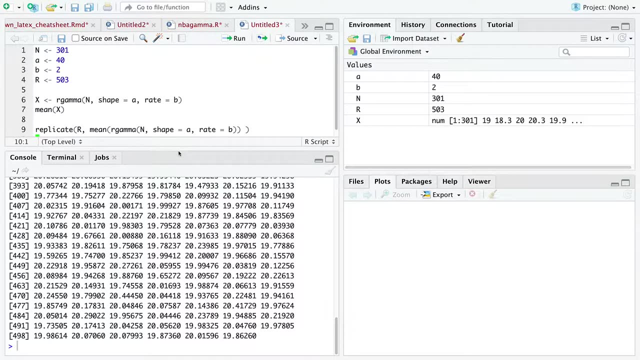 if I build that in the line of code I'm going to use~. all right, I'm going to do that. So I've kind of pulled this down to before, when it was anything like 27,. I've created this button profile here. 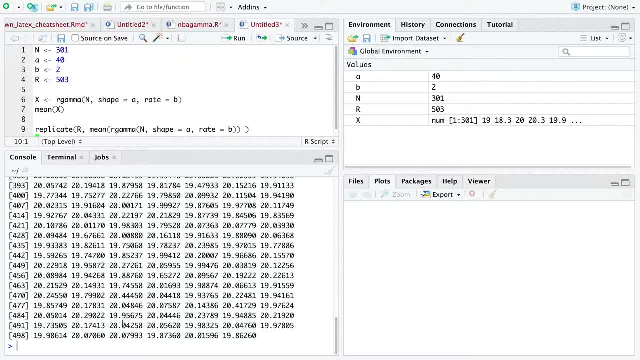 we're still going to prop it up and it's going to become 汬 higher. Okay, so now we're not going to bring up ministering here with 301 observations, within each mean, a rate of A and a shape of A and a rate of B. 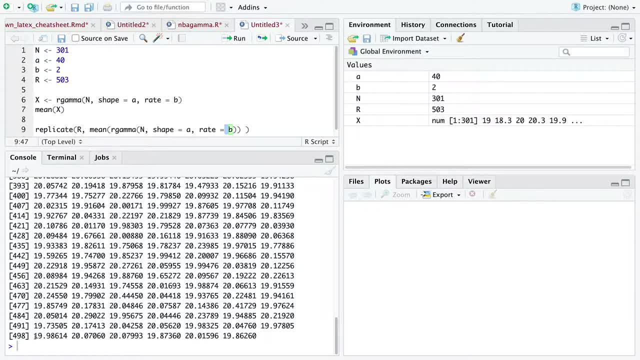 It's hard to see there is 503 of these, but indeed this 498 says: here is your 498th element, 99th, 500th, 1, 2, and 501.. Now, the thing to notice is that all of the means are really close to. 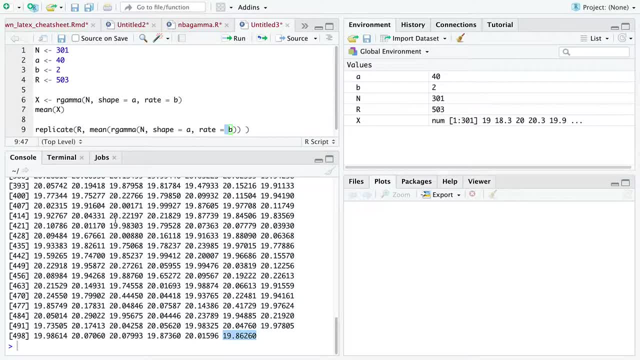 40 over 2, 20, because each mean is an estimate of the expectation A over B. So all we really have to do here is make a histogram. Here. let's stop doing too many parentheses and we'll break up the code into multiple variables. 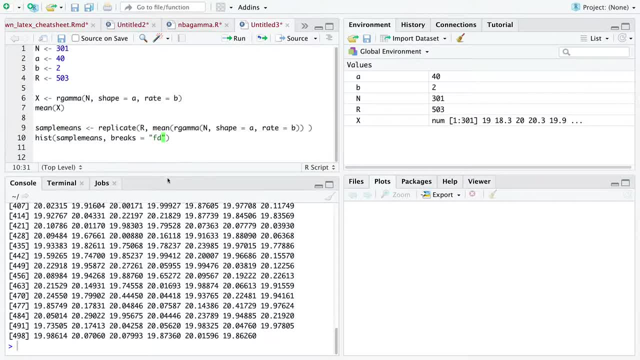 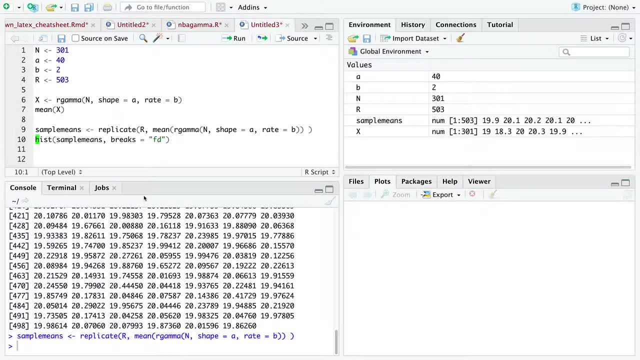 and I think that helps the eye read what's going on. So all we're going to do is run this line of code again, store it into a vector named- sample means, because the vector names what it holds- and then make a histogram using breaks equals FD. 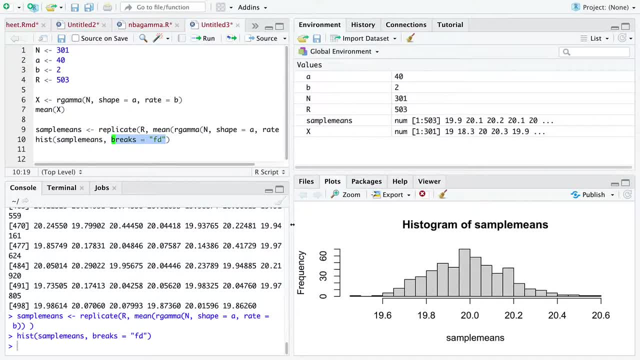 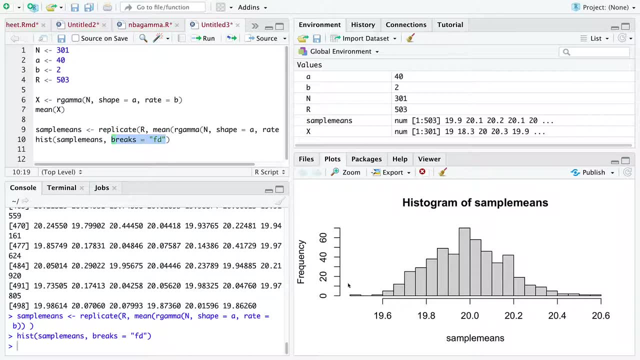 This is not necessary, but I like it because F Friedman and D Diaconis are two mathematicians from California And here is a histogram that I hope you see. that is approximately normal. it's got this kind of nice, almost symmetric shape to it. 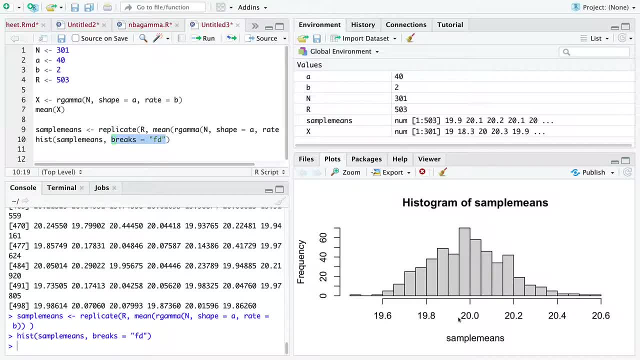 even though there's a few little asymmetries here, and it's centered at A over B, indeed just like it should be. So now the key takeaway is: it doesn't matter which distribution you sample from here or here, what you're going to get. 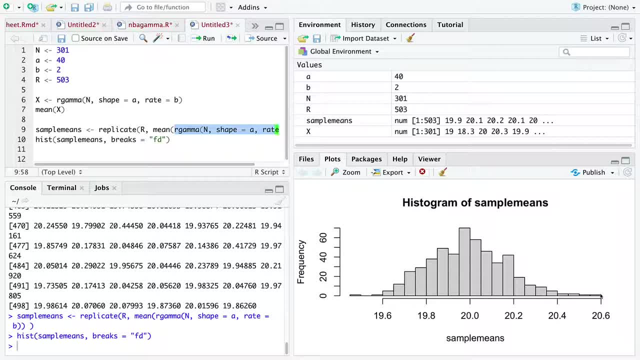 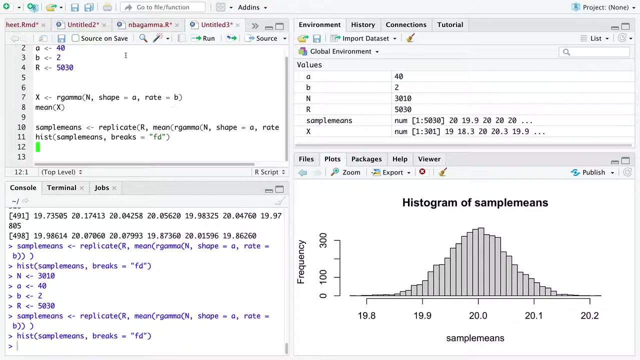 from the histogram of sample means indeed looks nearly normal, especially as these numbers and and R get bigger. this is going to look more and more normal. So we could repeat this process all over again, by just creating bigger sample sizes and claiming: you have more friends. 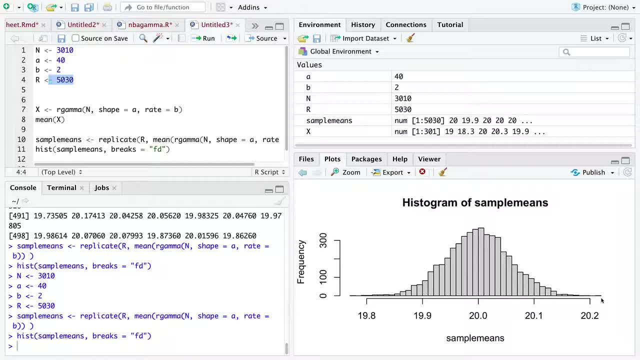 And indeed the sampling distribution we get out is normal. Now, remember, this week is a lot about exploration on your own, so what you should do is pick either a different distribution to sample from- and let's get rid of this- either a different distribution to sample from, right here.